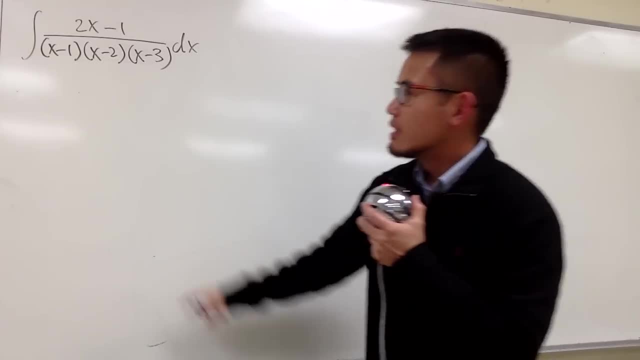 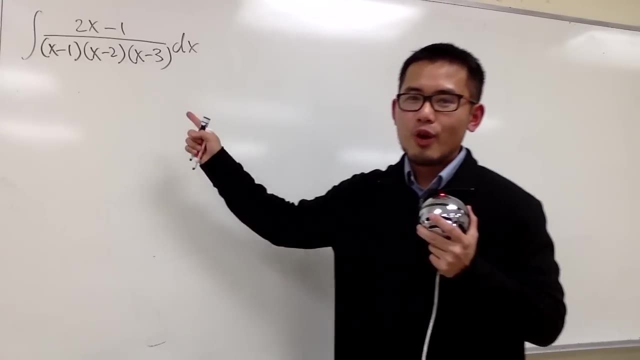 So we can go ahead and do the partial fraction And you see that all the factors in the denominators, they are all linear and they are all different. Therefore we can use partial fraction by the cover-up method. So first let's go ahead and set this up. 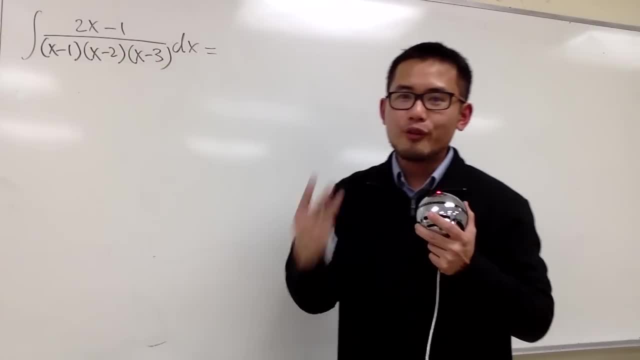 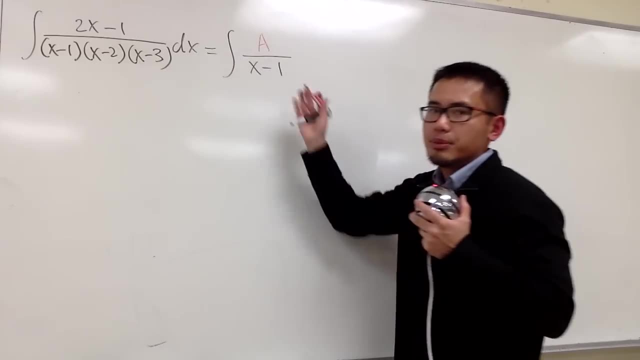 We know this right here can become 3 little fractions, right? So this is going to be the first one: x minus 1.. On the top we just have a constant and let's put on a, And then for the second one, we know the denominator will be x minus 2.. 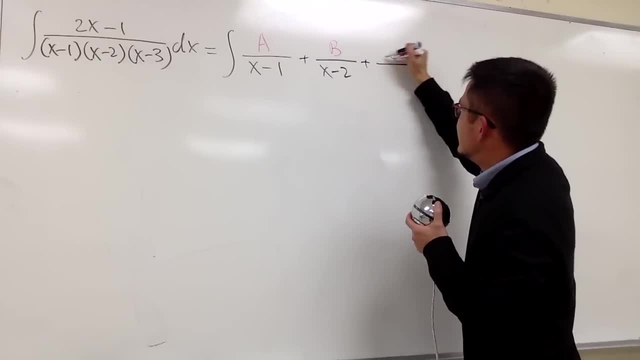 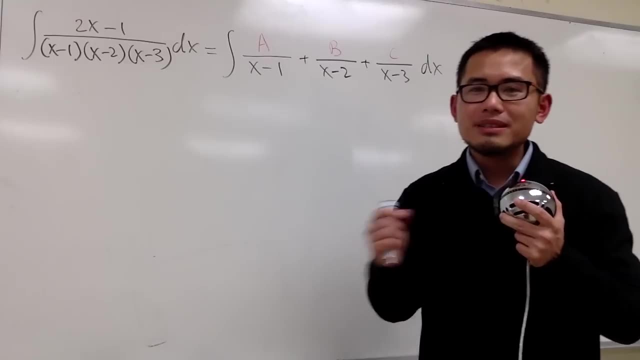 And let's put on b on the top. And the last one, it's going to be c over x minus 3 dx, And our goal at the moment is to find out what's a, b, c right, And I'm going to show you guys with the cover-up method. 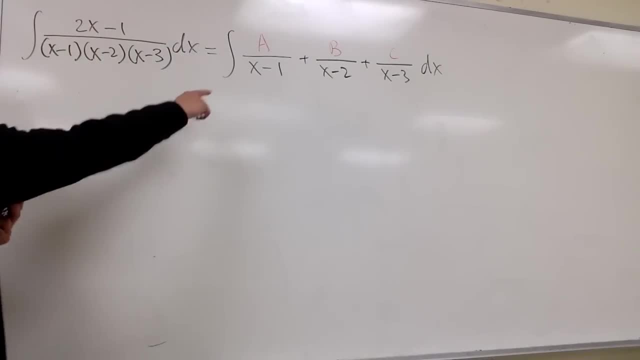 Okay, And this is the cover-up method And this is how we are going to do it. So I want to find out a first for you guys To do. so. you see that the denominator for a is x minus 1, right. 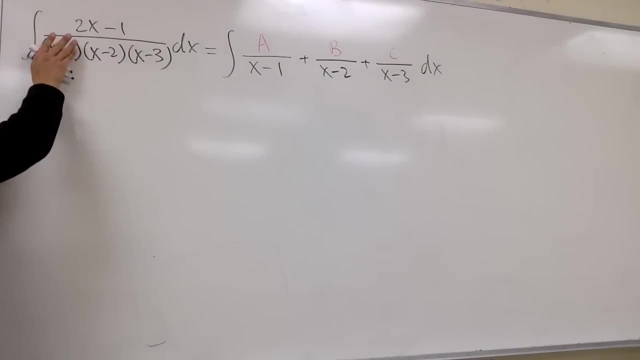 I'm going to go to the original. I'm going to cover the same denominator. This is what I'm going to be looking at. Okay, And let me write it down right here for you guys. a is going to be right here. I have to remember to let x equal to a number. 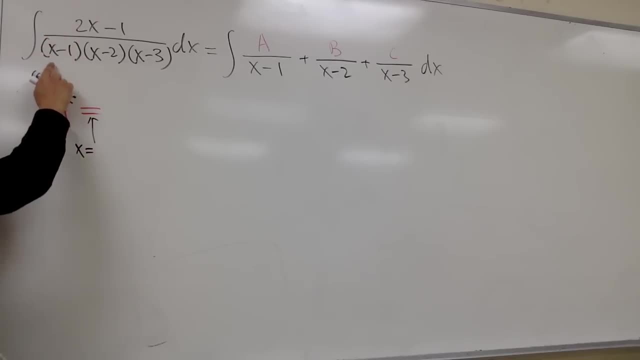 Okay, I covered this up. You have to ask yourself how can you make x minus 1 equal to 0?? Well, pick x is equal to 1, right? So let me pick x is equal to 1, and I will plug in 1 into the rest of this. x, right here. 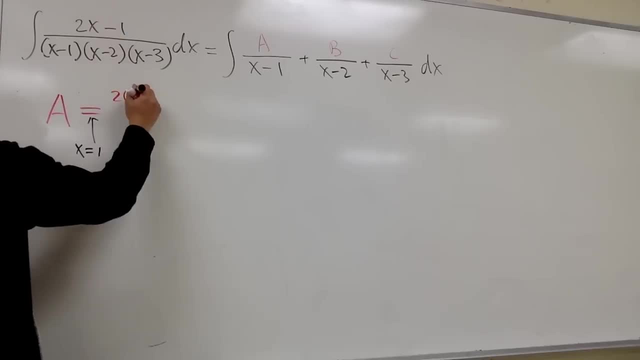 So a is going to be on the top. we have 2 times 1, and then minus 1, right Over. this is out already, because we covered it up. We will have 1 minus 2, like this: 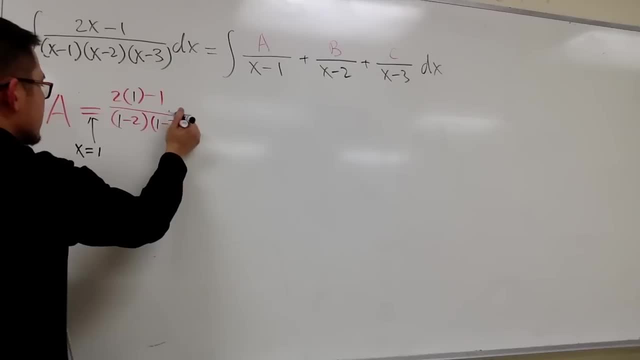 times 1 minus 3.. And now we can just, of course, work this out On the top: 2 times 1 is 2, minus 1 is just 1.. Over 1 minus 2 is negative 1,, 1 minus 3 is negative 2.. 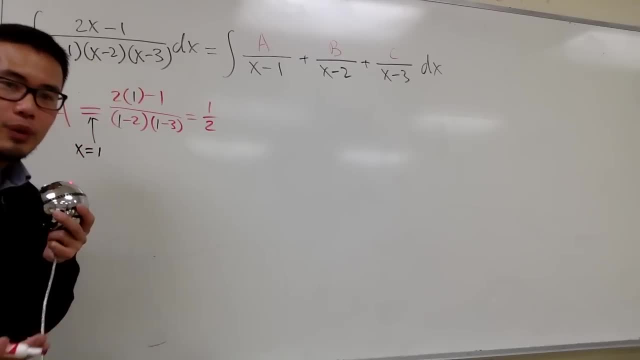 Negative 1 times negative 2, we have positive 2.. Therefore, we know a is equal to positive 1 half. And now let's go ahead and do the same for b, For b right here, this is going to be. you see, the denominator for b is x minus 2.. 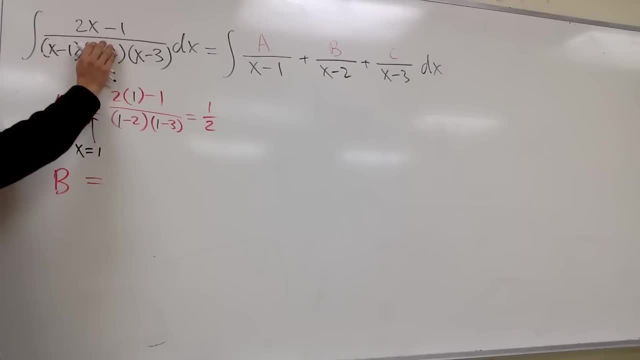 That means I have to come here, cover this up. and how can I make x minus 2 equal to 0?? Well, let's go ahead and let x equal to 2.. And now plug in 2 into the rest of this x, right here. 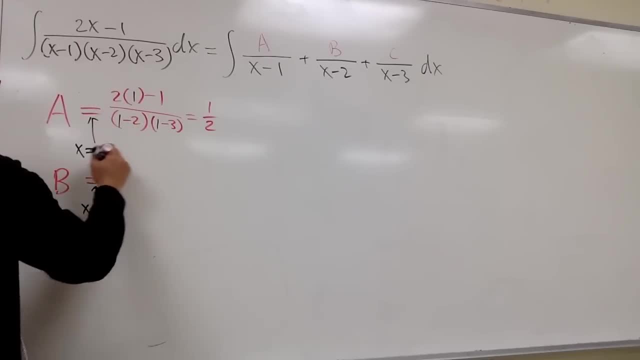 So we will have 2 on the top times, the x, which is 2, and then minus 1, right Over 2 in this x, we have 2 and then minus 1.. This is out already, and then we plug in 2 into this x. 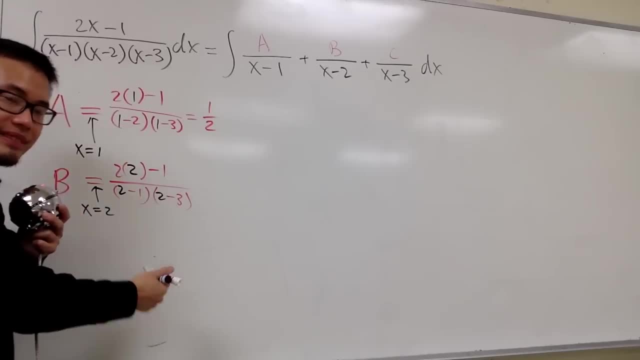 so we will have 2 minus 3, like this. And now, of course, let's just go ahead and work this out: 2 times 2 is 0.. 4 minus 1 is 3.. Over on the bottom, 2 minus 1 is 1.. 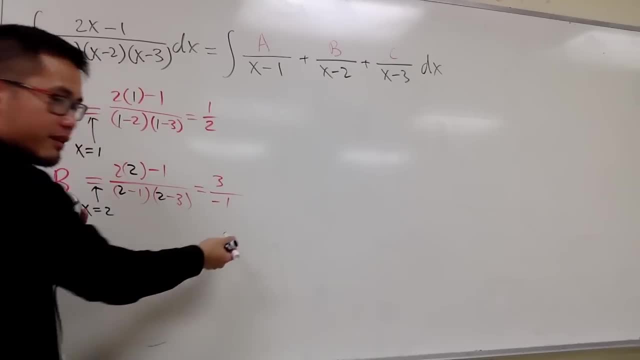 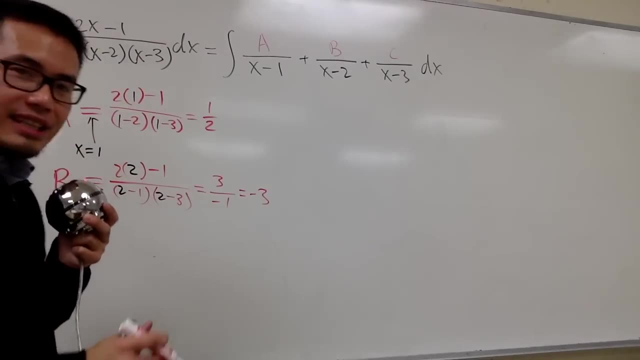 And then 2 minus 3 is negative 1, so this is what we have right, And at the end you see 3 over negative 1, this is just negative 3, like that Last one for c. 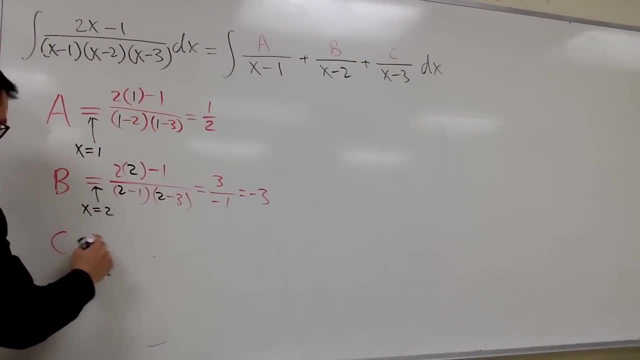 Okay, I'm going to cover this up right, And you see c is going to be. I have to let x equal to. how can I make x minus 3 equal to 0?? 3, right. So let x equal to 3.. 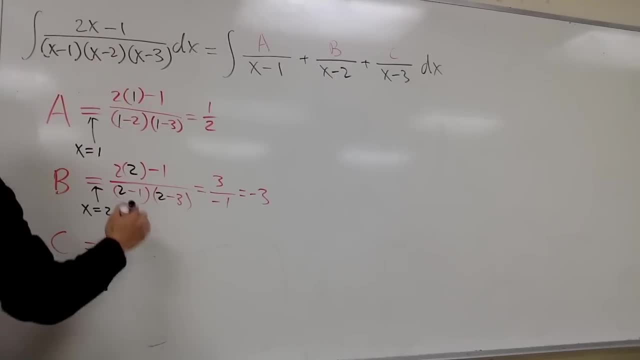 And plug in 3 into this x right here, So we will have 2 times 3, and then minus 1.. Over, and then this right here will be 3, so let's put that down And then minus 1, times 3 right here, and then minus 2.. 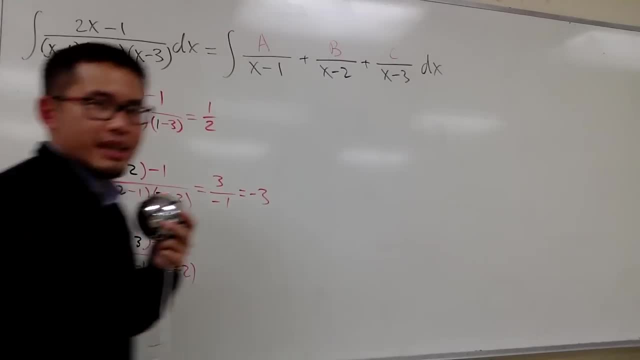 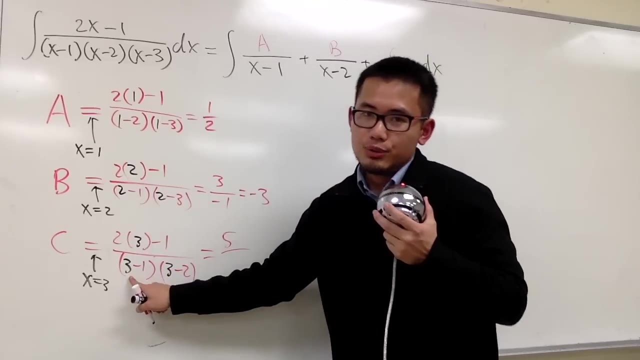 And this is out already, because we covered it up And now you see this right here. just work this out: 2 times 3 is 6, minus 1 is 5.. Over 3 minus 1 is 2.. 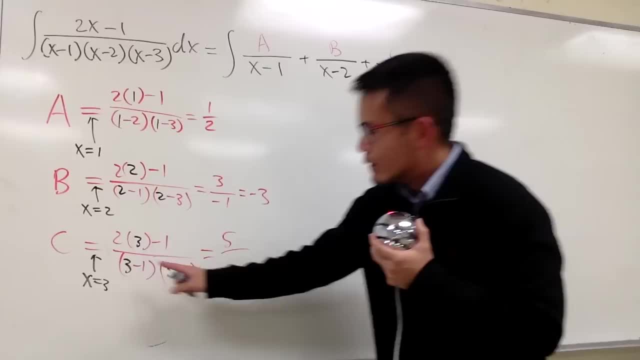 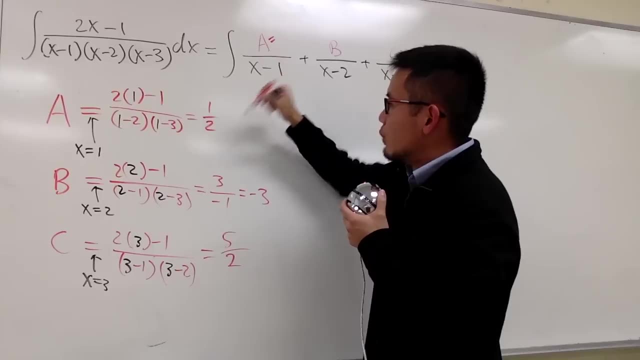 1 is 2.. And then 3 minus 2 is 1.. 2 times 1 is, of course, just 2.. So these are the a, b, c values. And now you see, a is 1 half. 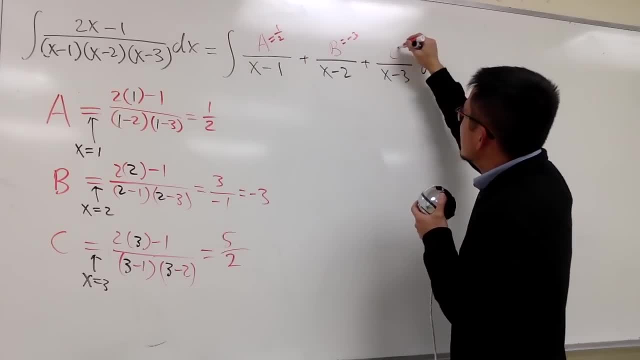 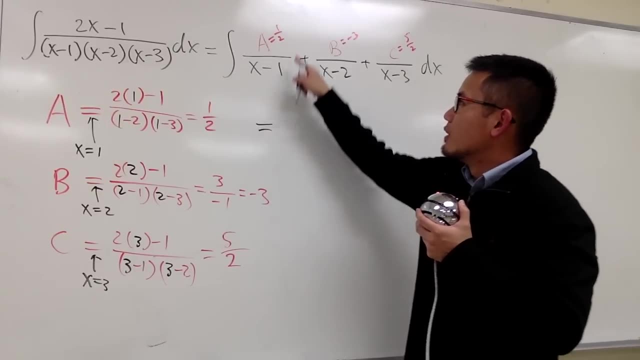 b is negative 3. And c is 5 over 2. And that's the partial fraction by the cover-up method. So at the end let's just put down the constant multiple first and then let's integrate, right. 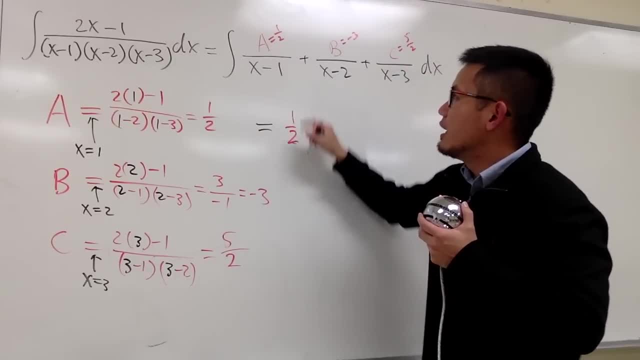 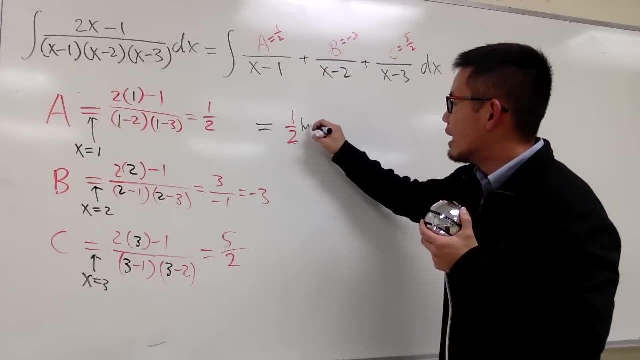 So for the 1 half, we can just put that down. so we have 1 half. And to integrate 1 over x minus 1, and this is x to the first power, it will be ln absolute value of x minus 1.. 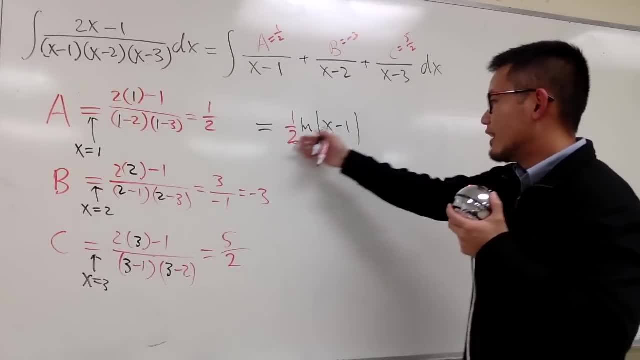 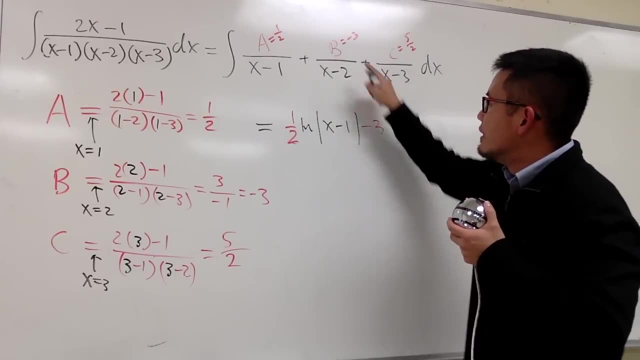 And the derivative of x minus 1 is just 1.. So dividing by 1 doesn't matter. This is what we have for the first term. Next, this is minus 3.. Let's put that down first. And then this is: we have to integrate 1 over x minus 2.. 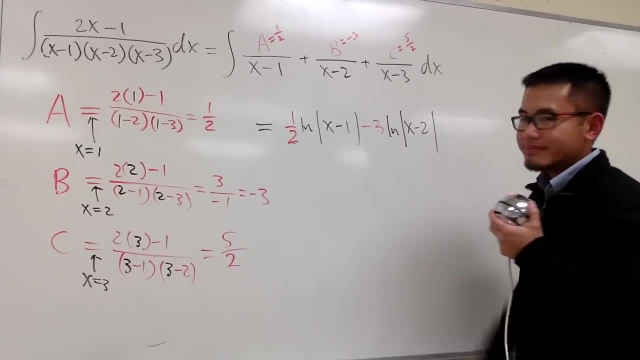 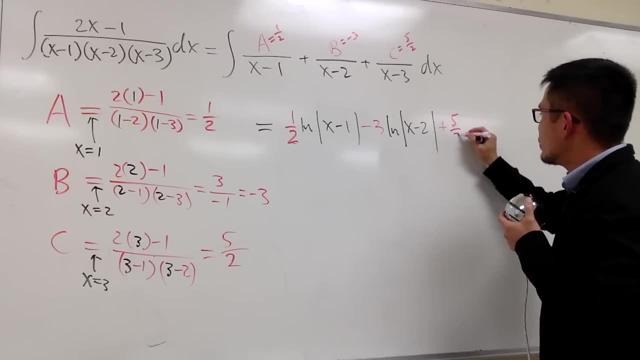 We'll end up ln absolute value, x minus 2.. And the last one, 5 over 2.. You know that's the constant multiple, so let's write that down. This is plus 5 over 2. And we have to integrate 1 over x minus 3.. 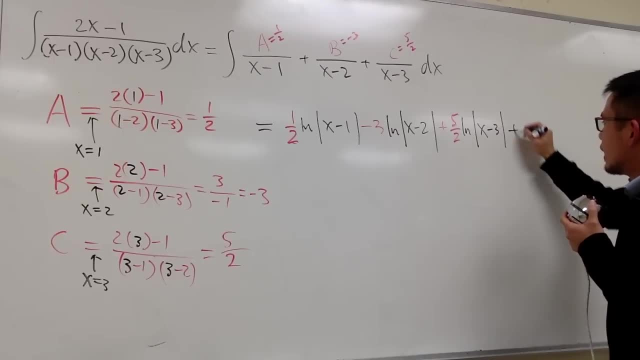 We will end up ln, absolute value x minus 3.. And then we are all done. So let's put a plus c. This right here. That's it. 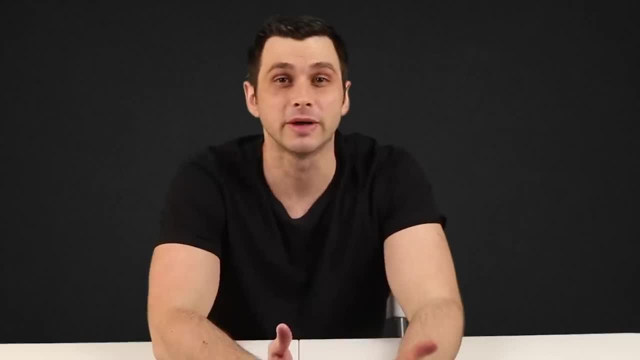 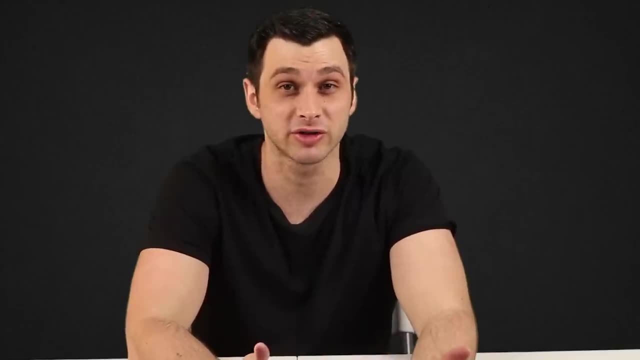 This video is sponsored by Brilliant. Let's just get to the point. Why do we learn differential equations? Because they are the equations that describe how nature works. The universe one day said, boom, here's a bunch of stuff. And we said, cool, how's it all work? 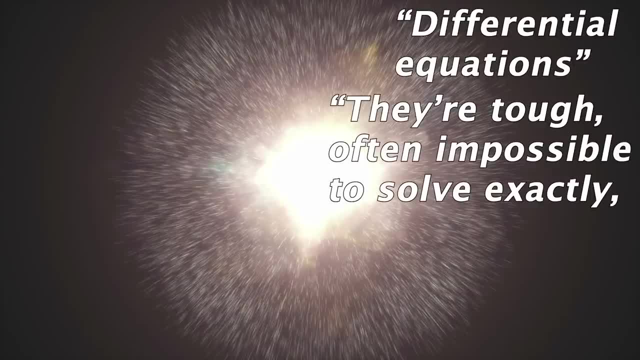 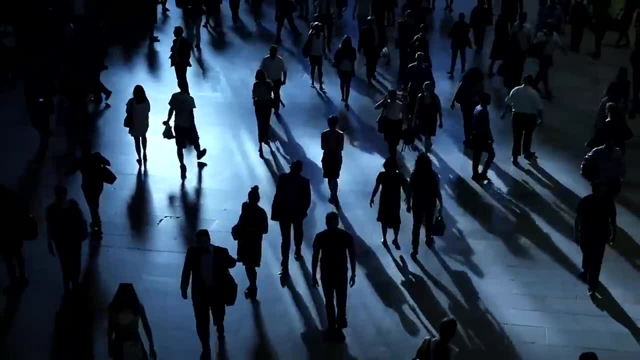 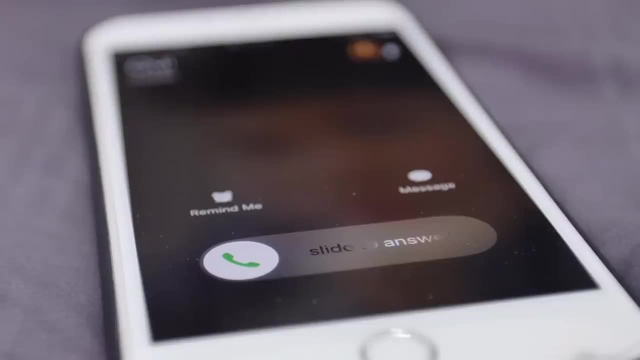 And the universe said: differential equations. They're tough, often impossible to solve exactly, but you'll eventually get some cool stuff from them. Modeling how a population will grow involves differential equations How any fluid moves, differential equations Electromagnetism, which is how phones radio. 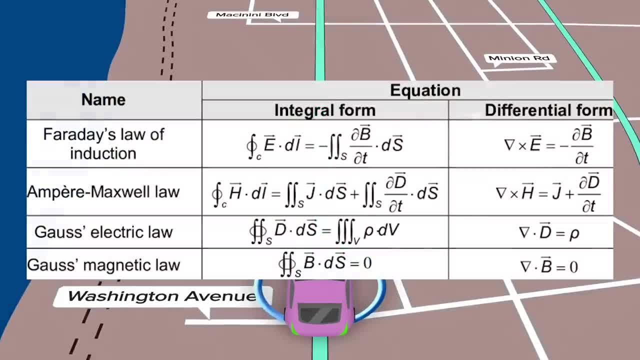 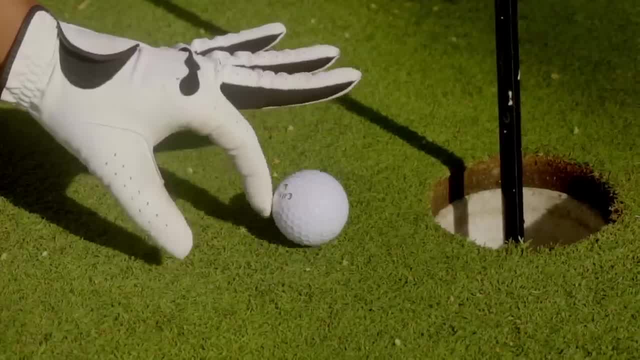 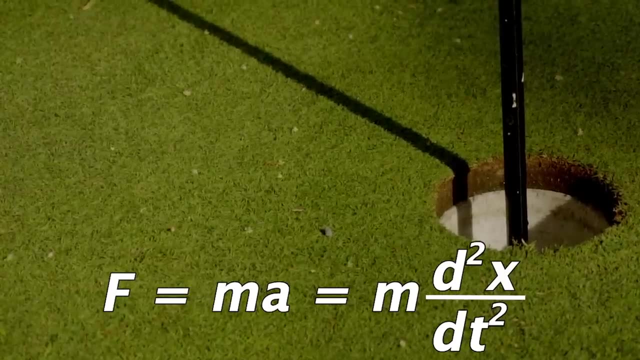 Wi-Fi and GPS all work. Not one, but four differential equations, known as Maxwell's equations. There's electric circuits, and even if something touches something else and thus exerts a force, differential equations are used to describe the motion. If there's no physical contact, like with orbiting bodies,